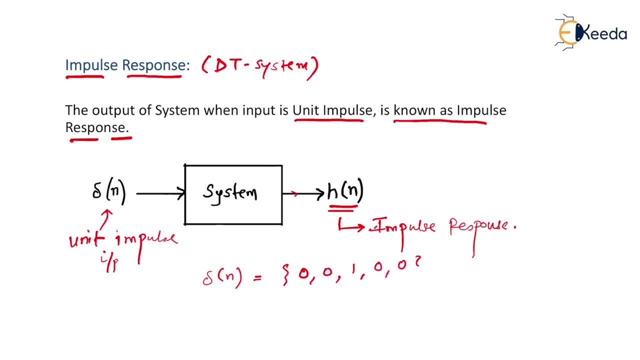 sequence. we write it this way. We know that an arrow mark indicates the sample position at n equal to 0. So when I start drawing this del of n, it is having amplitude 1 at n equal to 0, and it is always 0.. 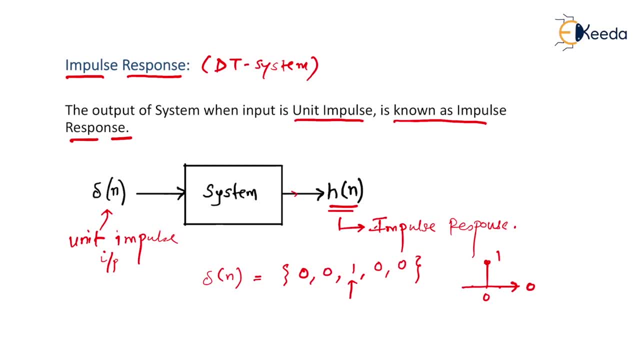 Otherwise, am I right? So this is the kind of input. if I apply it to a system, then the output given by the system or response given by the system is called as impulse response, that is, response given to an impulse input. Now the question is why. 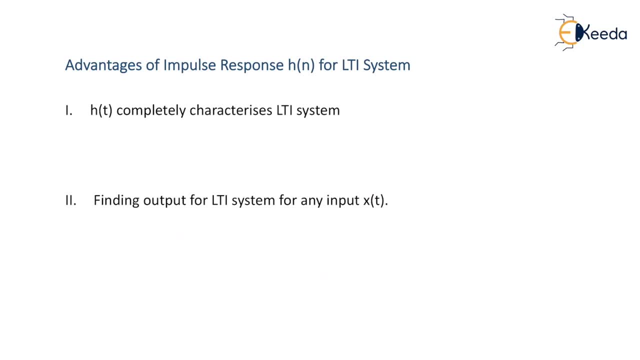 to apply an impulse input and thereafter, once you apply an impulse input, the output that you get is what we called as an impulse response, and why impulse response is very, very important for us. So now we are going to see advantages of impulse response. First of all, you have to understand that initial output is an 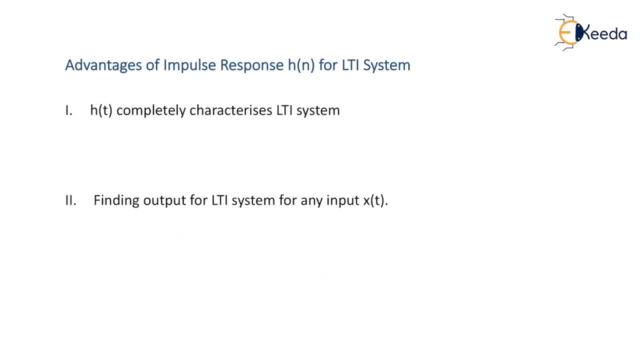 quantum. whenever divided input is fois minus sigma n kost n próximian n ber Kafkaanın will be used. No key LED will be given to the second saying. but this is the reason. response H of n, specially for LTI system. So when I say LTI system, it means it consists of two. 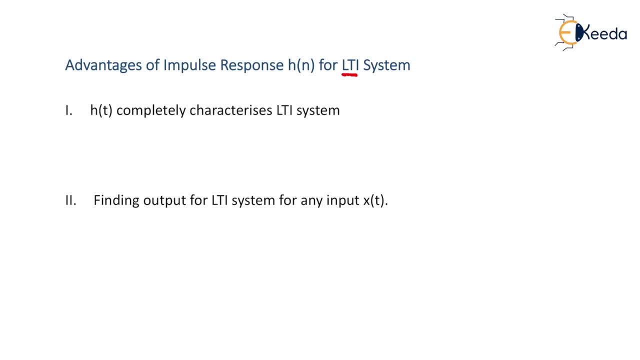 inherent properties. that is, it is linear as well as time invariant system. I'm sure you must have seen the previous videos where I have made you understand very clearly what are linear systems and what are time invariant systems. So linear systems are those systems which follows additivity. 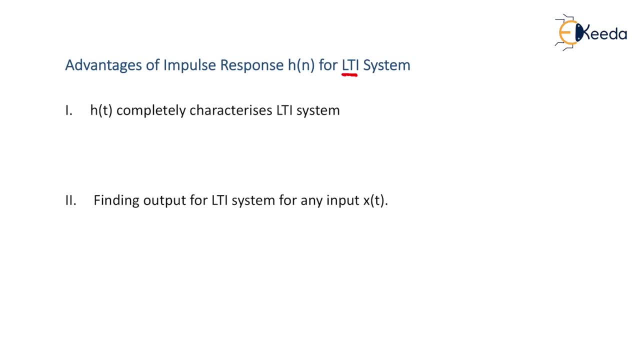 as well as homogeneity principle, whereas time invariant systems are those systems which can be described this way: For example, if you apply input as x of t and let's say output is y of t, then if you delay the input, let's say by t, naught amount. so this time let's say you are applying x. 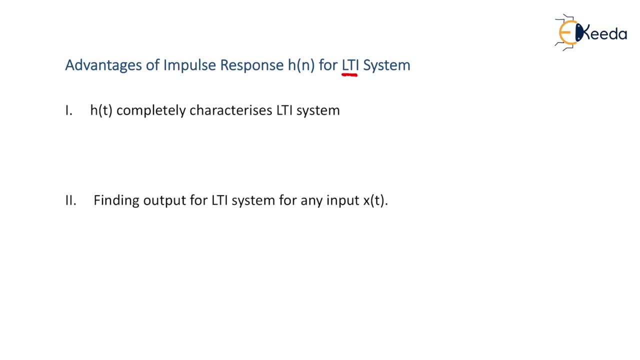 of t minus 1, then output must be y of t minus 1, meaning that the quantity by which you are going to delay your input, by same quantity your output should also get delayed. In fact, time invariant systems are those systems whose properties do not change with respect to. 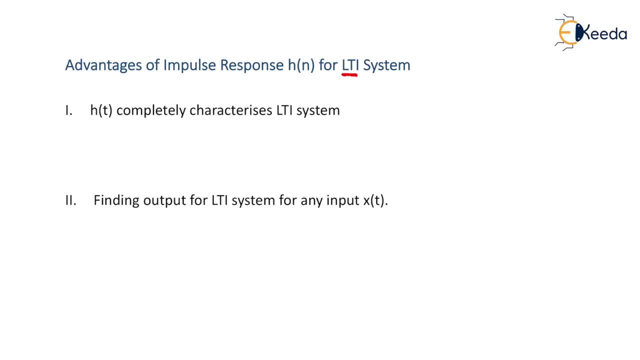 time they remain same. So why do we study LTI system? because LTI systems are considered to be ideal systems. Let me tell you, when you get into practical systems, they are quite non-linear, as well, as they could be time variant system also. But then we study non-linear systems and time. 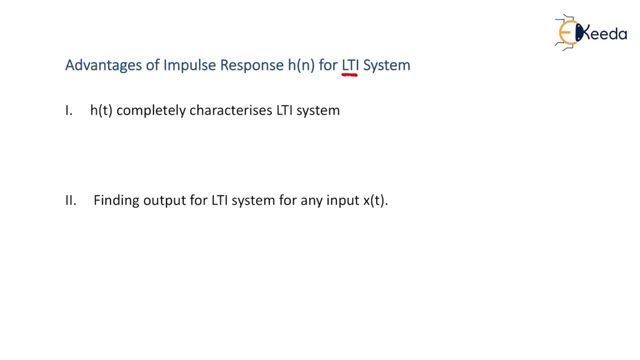 variant system. when we learn advanced control system, or whenever you will go to masters there only, you will be studying those systems, that is, non-linear systems as well as time variant system. According to Gates syllabus, we are going to concentrate only on those systems which are 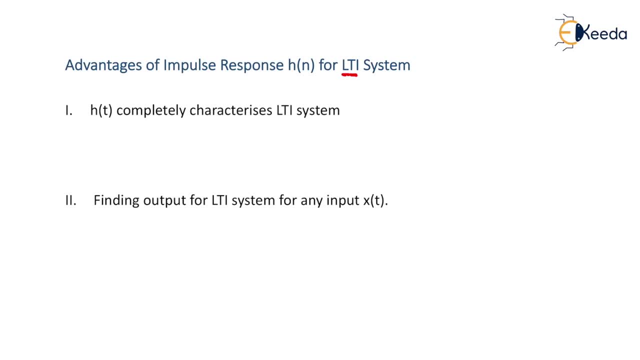 linear in nature as well as time invariant in nature. So a system with both properties is called as LTI system. So the discussion over here is limited to LTI system only. So first of all you can see h of t completely characterizes LTI system. So what is meant by it? completely characterizes. 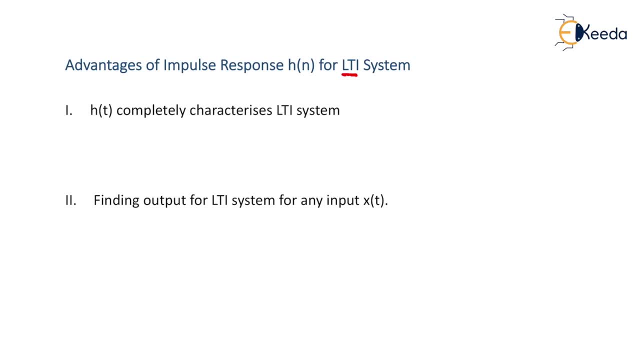 LTI system means h of t is going to tell you a complete behavior of the system. So first note that it tells you about behavior of the system. You also understand the causality of the system, means if the system is causal or non-causal. So 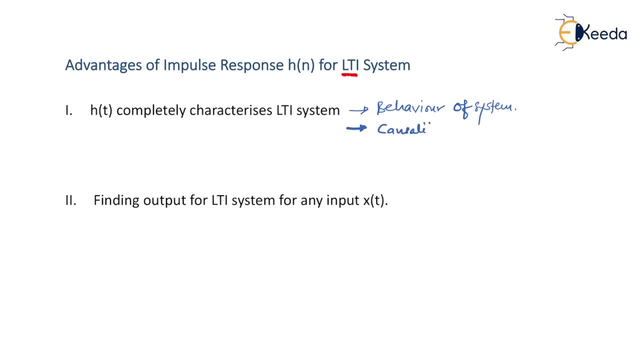 you understand a causality. also, Along with the causality, you understand a stability of system. You understand whether systems are static or dynamic. Also, from h of t you can determine whether the system is invertible or non-invertible in nature. So you understand whether your systems are invertible or not. So these many things, these much. 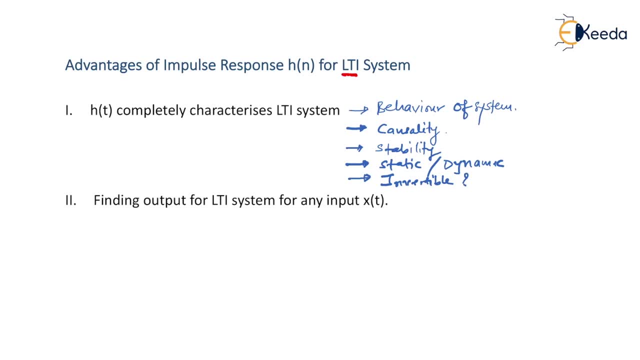 information is given by alone h of t. So for a particular LTI system, if h of t is known to me, I can characterize a complete system, whether it is causal or non-causal, whether it is stable or unstable, whether it is static or dynamic. also we will understand whether it is invertible or non-invertible in nature. see a single h of t. 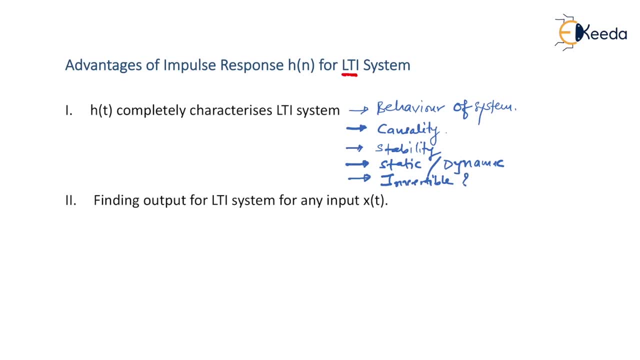 is going to tell you these many things about lti system. yes, when it is non-lti system, then only h of t is not enough. we require other parameters also to characterize that system. but when it comes to lti system, h of t is enough to tell about a system that is in and out about the system. 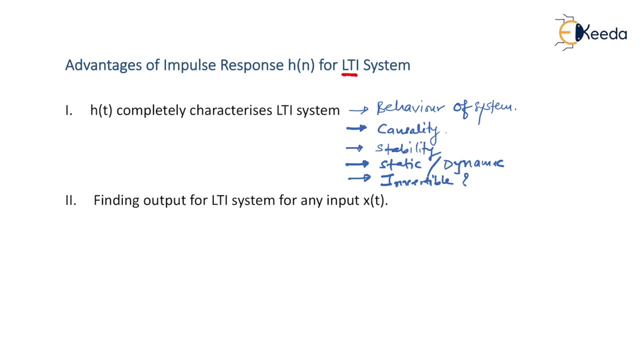 the second advantage says finding output of lti system. for any input, x of t. okay, for example, let's say if h of t is known to you, now you know that what is h of t. h of t is called as impulse response. so for a particular system, let's say: if h of t is known to me, and let's say you are. 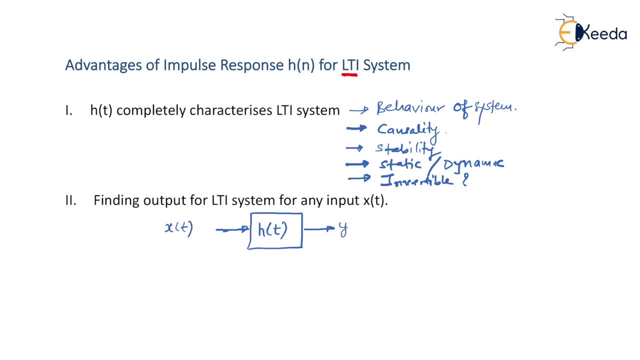 applying some input- x of t- then you can determine what is y of t where y of t is known to you, and you can determine what is h of t is known to you, and you can determine what is x of t convolved with h of t, because x of t is an input that we are applying from our 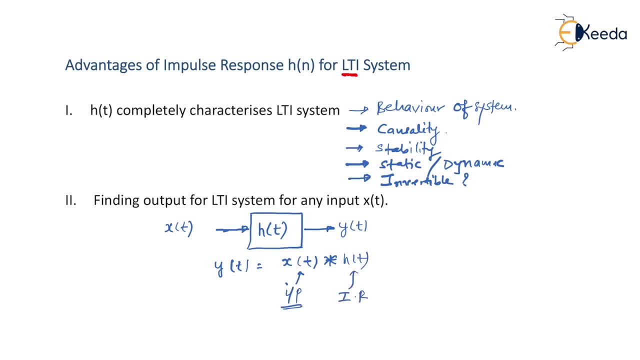 interest. h of t is an impulse response. it is in advance, let's say, known to me. so it is quite possible for us to derive y of t mathematically by using: y of t is equal to x of t convolved with h of t. now the sign over here, that is an operator called as a convolution operator. 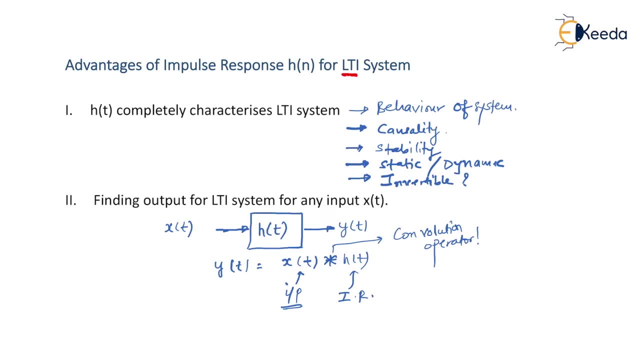 right now i have used notations as: x of t, y of t and y of t is equal to x of t convolved with h of t. it clearly indicates i'm talking about a continuous time signal system, right? but yes, of course you can have the same property in discrete time sense also. so instead of x of t, you will have x of n. 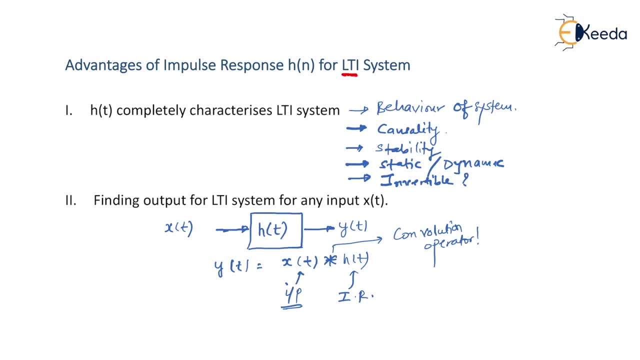 instead of h of t you will have h of n, and instead of y of t as output, you will have y of n, and relation remains same, that is, y of n will be x of n convolved with h of n. so it really doesn't matter whether you are working with 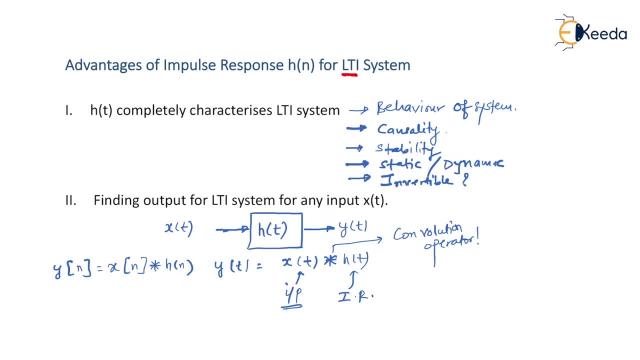 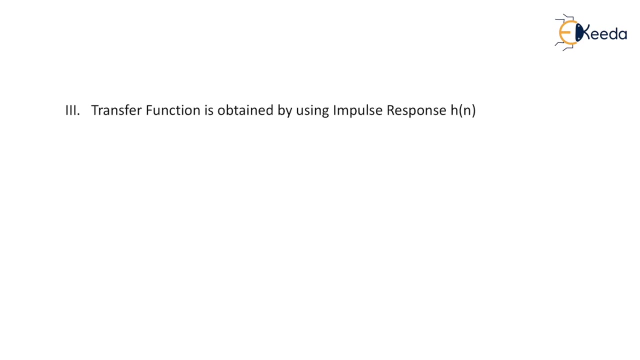 continuous time system or discrete time system, relation between input, impulse response and output remains same. so what it means that if impulse response is known to you, it is possible for you to find the output for any input right. third and very important conclusion: that transfer function is obtained by using impulse response only. 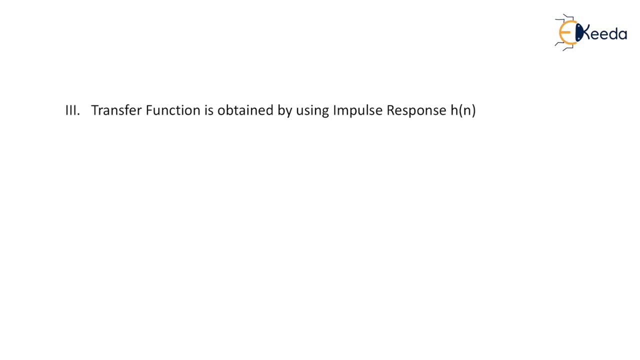 if you have done control system, you must have learned about transfer function, so that transfer function is what we called as h of s. so if you have an impulse response, let us assume h of t. if you take a laplace transform of this, you get h of s. so h of s is called as a transfer function. 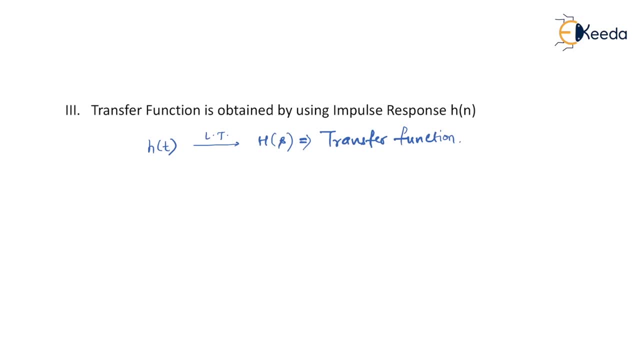 and using those transfer functions- let's say if it is transfer function of a closed loop control system- you can determine the closed loop pole's location and from that also you can identify whether system is stable or unstable. right also you can characterize the system, i mean you can find limitations on the gain of the system, for which system will be stable by using 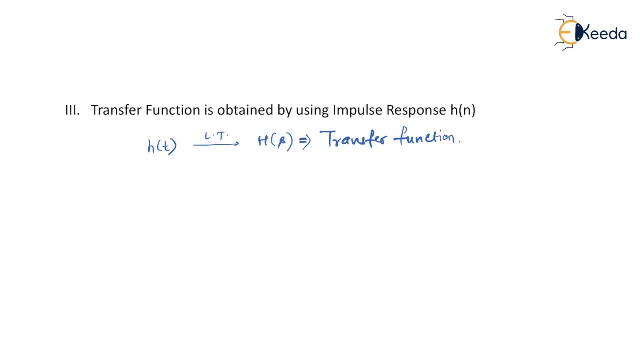 many tools, like a root locus and all, but for that you must have a transfer function. and if you want a transfer function, it is basically obtained by having a laplace transform of h of t. only suppose, in this h of s, if you, let's say, substitute s equal to j omega, then it becomes h of j omega. 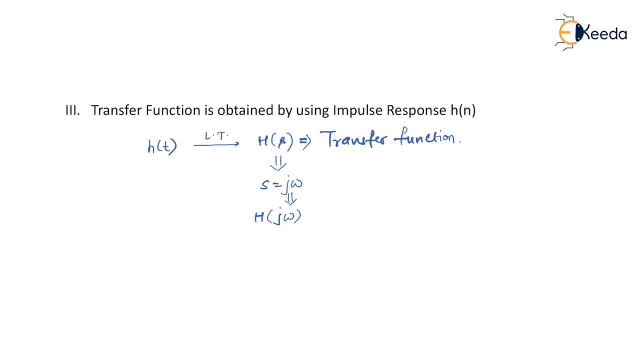 so this is the another way to get h of j omega, by using substitution as s equal to j omega or from h of t. also, you can get h of j omega by having a Fourier transform. so Fourier transform is the another tool by which you can get h of j omega. and the use of h of j omega is to know the frequency response of the system. 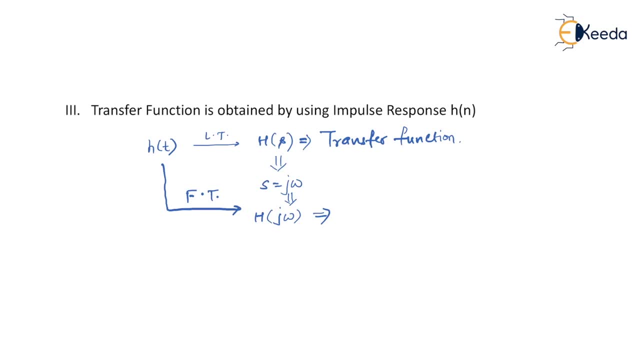 So h of j omega is used to study frequency response of the system. using this frequency response you can have two categories, that is, a magnitude response and a phase response. so magnitude response tells you how magnitude of the system is changing with respect to frequency and how phase is changing with respect to frequency. 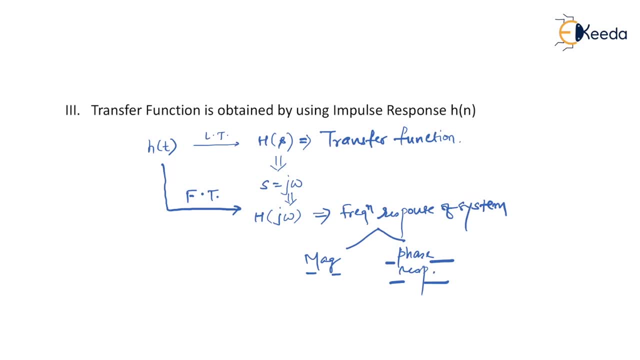 it is obtained with phase response. so, as you can see, just one response, that is, impulse response, has so many advantages, right? so studying impulse response is very, very important, because if you don't know what is impulse response, then it is impossible to have transfer function h of s or 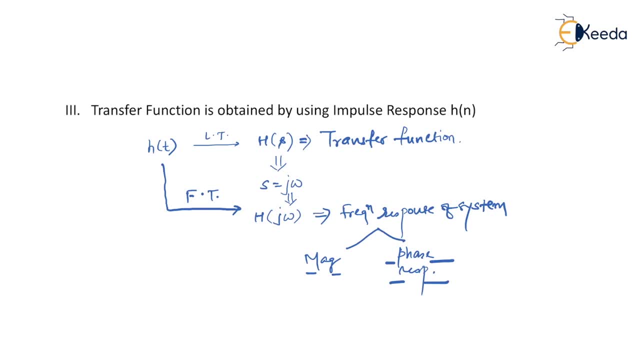 it is impossible to have h of j omega, which makes you capable to study frequency response of the system. so now read the question: find mathematical representation of x of n to the power of h of s. So what is the significance of the arrow mark? So this is the sample present at n equal to 0.. 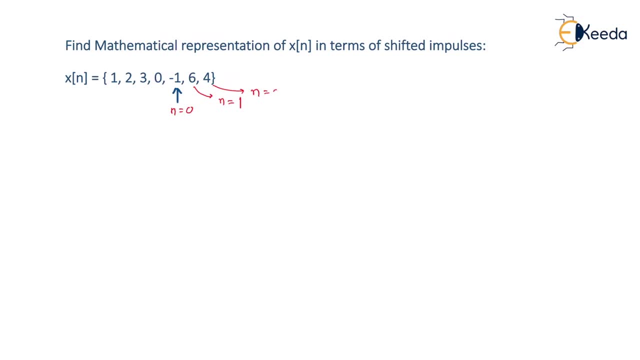 6 is present at n equal to 1.. 4 is present at n equal to 2.. then zero means there is no amplitude present or zero sample present at n equal to minus one. This is present at n equal to minus two. 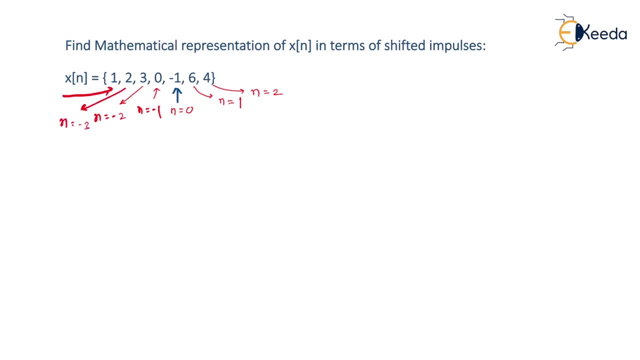 present at n equal to minus 3, and finally, this one is present at n equal to minus 4. is that right? so now to express a mathematical representation of x, of n in terms of shifted impulses, we need to do a little exercise. so what i meant. suppose you have a random sequence like this. let's say: 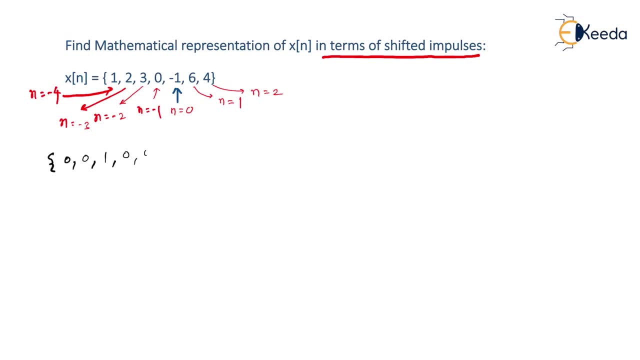 0, 0, then you have 1, then you have 0, 0 here. and let's say, if i'm showing an arrow mark here, i'm sure you must have recognized that only at n equal to 0 a signal is present having magnitude equal to 1 or amplitude equal to 1, and it is equal to 0 when n is not equal to 0. so only at. 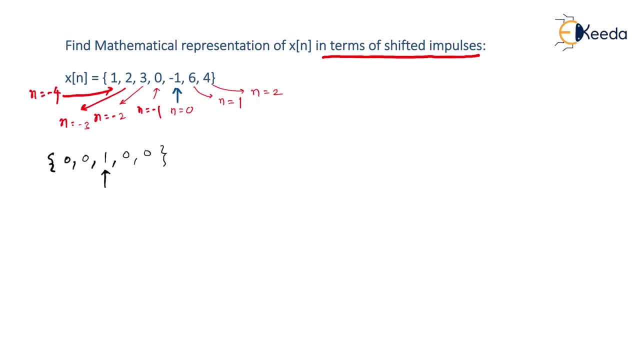 n equal to 0, if some sample is present, then this is of course known as what it is known as an impulse input del of n, because we know that del of n is equal to 1 only at n equal to 0. if some sample is present, then this is of course known as what it is known. 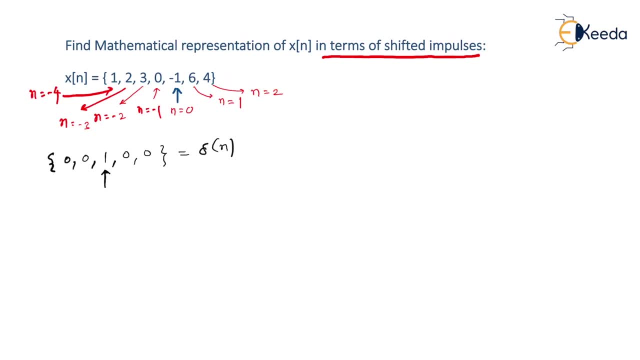 only at n equal to 0, and del of n is always 0 when n is not equal to 0. now suppose, if i modify this too, and let's say we have an arrow mark here, then what does that indicate? of course, now, only at n. 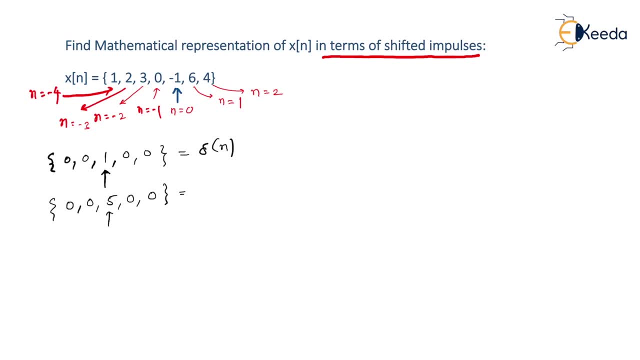 equal to 0. some sample is present having amplitude equal to 5, right? in that case you can write it like this: 5 del of n, because ultimately sample is present only at n equal to 0, but this time amplitude equal to 5. then you can say it is 5. 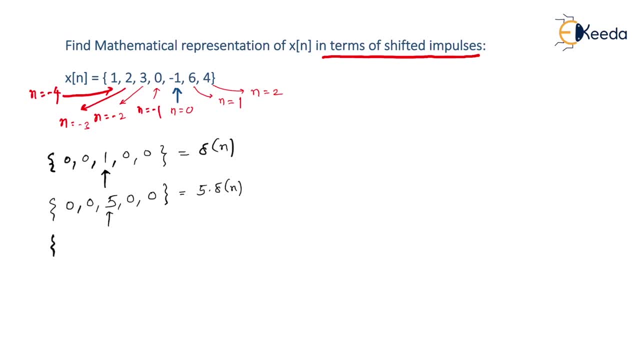 times del of n. now, for example, you have this kind of response or this type of input sequence and again, at n equal to 0, it is having amplitude equal to minus 2. then you can write this as minus 2 times del of n. is that right? 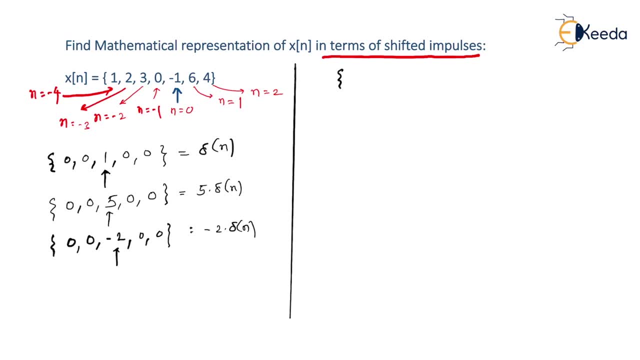 now, for example, we have this kind of response. now, what does that mean? an arrow mark indicates n equal to 0 position and this 1 is present at n equal to minus 1 position. is that right? so now you can express in terms of impulse input or in terms of impulse signal, like this del of n plus 1. we know that. what? 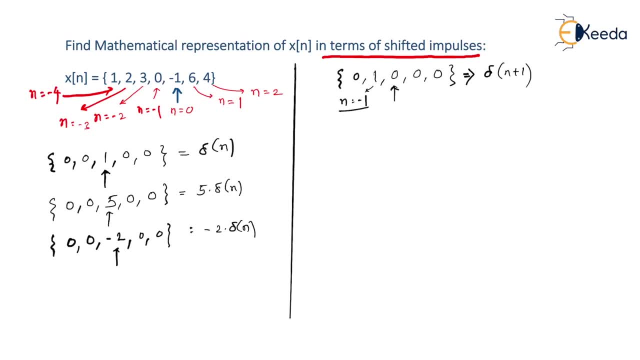 is meant by del of n plus 1. del of n plus 1 is the value of the impulse signal. like this: del of n plus 1 means an impulse present at n equal to minus 1 position. am i right? and again, since it has got amplitude equal to 1, i have kept coefficient equal to 1 only, so this is what we called as a. 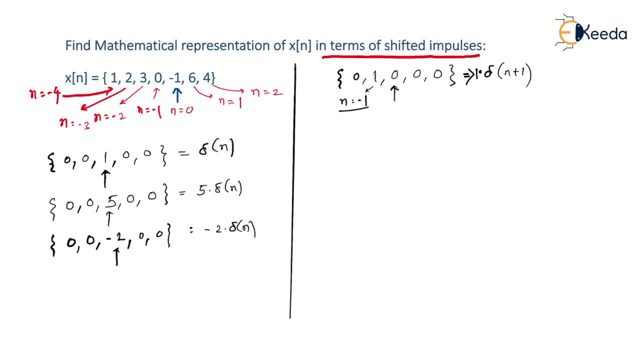 coefficient. so if the coefficient is 1, there is no need to write one pulse, for example. let's say we have this type of sequence. then how do we express this? we know that an arrow mark indicates it is a sample present at n equal to 0. is that right? 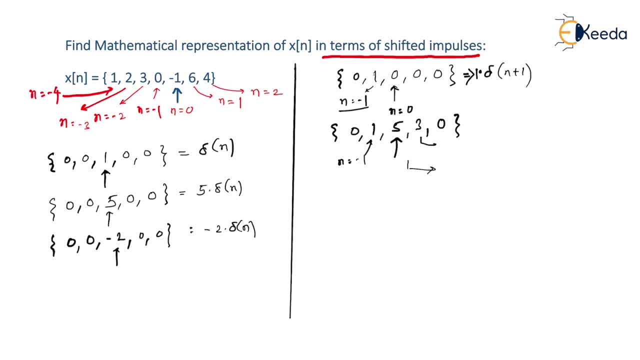 this is the sample present at n equal to minus 1 and this is the sample present at n equal to positive 1. so for n equal to minus 1 sample, we write it in this way: that is: del of n plus 1 is that right now. coefficient is 1, then at n equal to 0, sample position amplitude is 5. 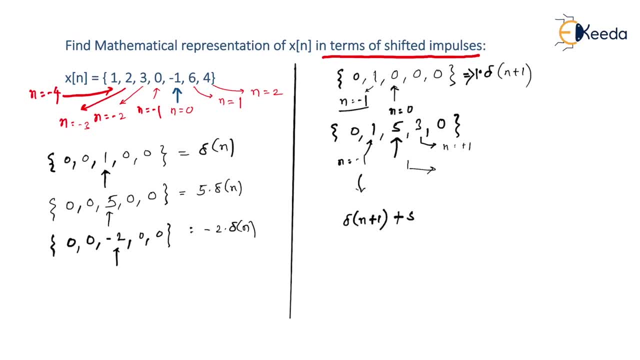 or sample, amplitude is 5 at n equal to 0, i can write plus 5 times del of n plus now for 3, i can write 3 times del of n minus 1, because this is a sample position having an amplitude equal to 3, present at n equal to plus 1, so i can write n. 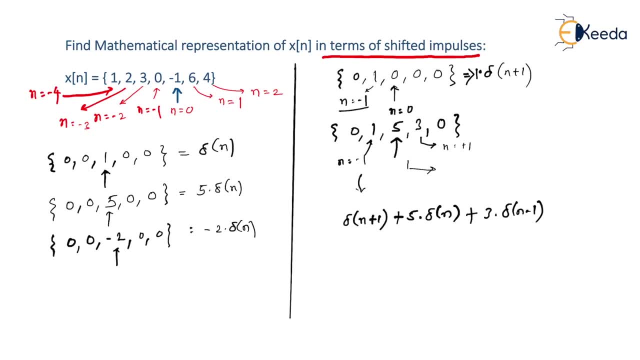 minus 1. so this is how, for a given sequence, we can express it in terms of shifted impulse input, because these are called a shifted impulse input, because this is what we called as an impulse, but this is called as a shifted impulse. this is also a shifted impulse. 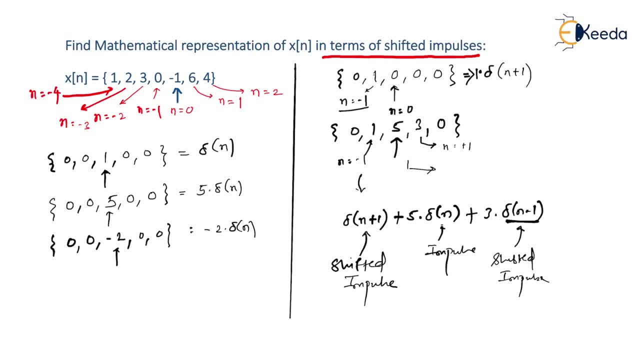 so this is shifted in the sense it is delayed by 1, and this is shifted in the sense it is advanced by 1, and this is present at n equal to 0. so this is only called as an impulse, meaning that if some sequence is given, i can express that sequence in terms of shifted impulse, input, summation together. 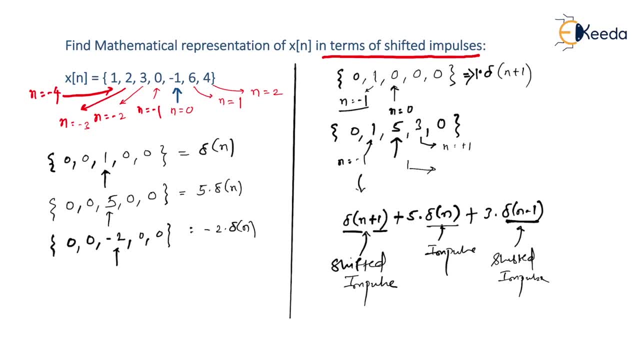 am i right? so now i'm sure it is quite easy to express this x of n in terms of shifted impulse input. so let us try that also now. so i'll be starting with extreme left. that is n equal to minus 4 position. so at n equal to minus 4 position, it is having signal magnitude or signal amplitude. 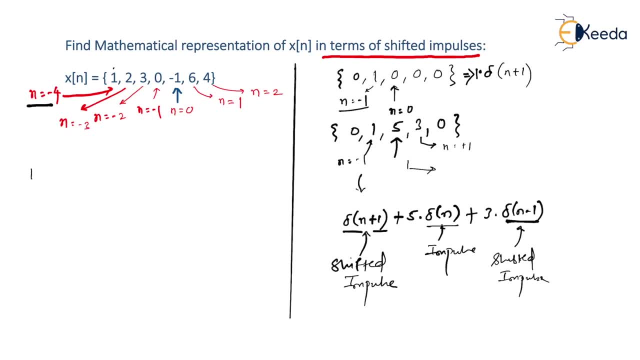 equal to plus 1, so coefficient is 1, so i can write 1 del of n plus 4. is that right? because if sample position is present at n equal to minus 4, you write del of n plus 4. then another sample having amplitude equal to 2. 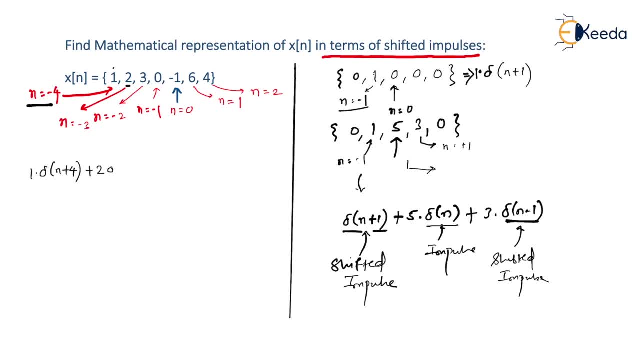 so you will say plus having an amplitude equal to 2 del of position, is n equal to minus 3. i supposed to write n plus 3. then you have to consider this sample, that is, having an amplitude positive 3, then coefficient is positive 3 present at n equal to minus 2 position, then i supposed to. 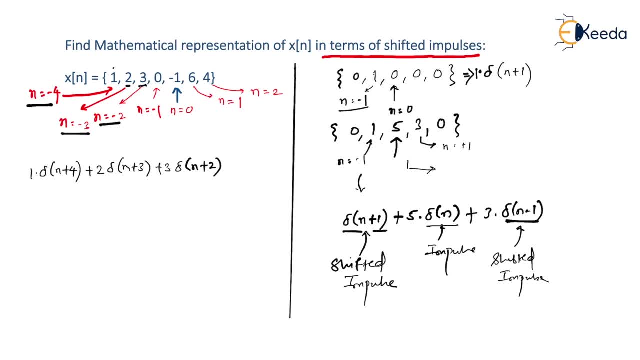 write del of n plus 2. after that you are having no sample. okay, when they say amplitude equal to 0, it means there is no sample present. at n equal to minus 1, it means the coefficient is 0. so you can write like this: 0 times del of n plus 1. but then it is quite not needed to write if the sample 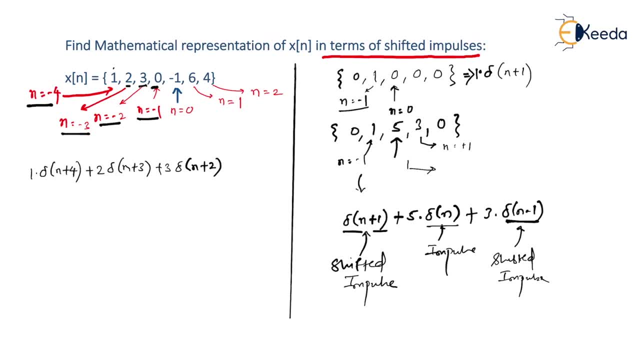 position is 0, so you don't have to express for a sample whose amplitude equal to 0 there. then i can write it for minus 1. so i can write minus 1. and minus 1 is present at n equal to 0, so i can say: 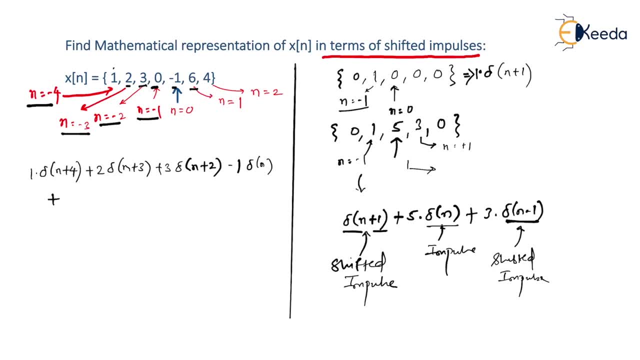 minus 1 del of n, then for 6 i can write plus 6. see, it depends upon the amplitude. if the amplitude is minus 1, i'm writing coefficient as minus 1. if the amplitude is plus 6, i'll write coefficient as plus 6. present at n, equal to 1 position. 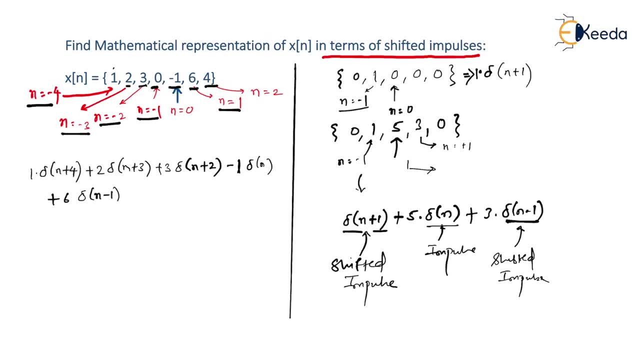 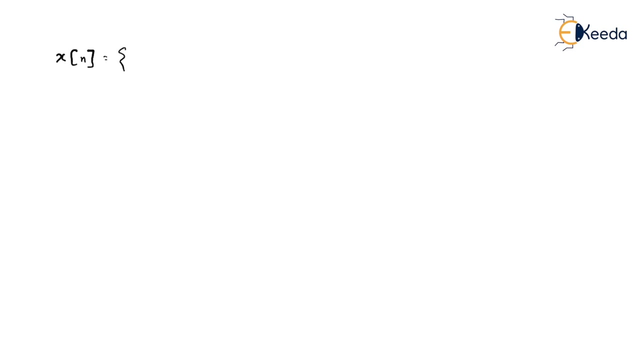 i supposed to write del of n minus 1 and last, having amplitude 4 present at n equal to positive 2, i supposed to write n minus 2. is that right? or else i can write it this way. so i'll take one more example. i'll conclude this. let me have another sequence, x of n as: 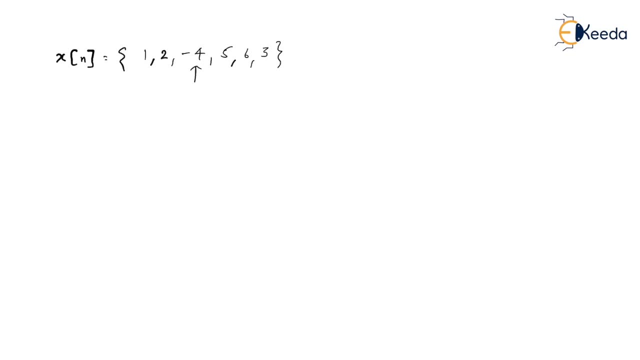 so let us try to express the given x of n sequence in terms of shifted impulse input. so now i'm sure it is easy for you. so this is the position at n equal to 0. arrow mark indicates it. this is n equal to 1, n equal to 2 and this 3 is present at n equal to 3. 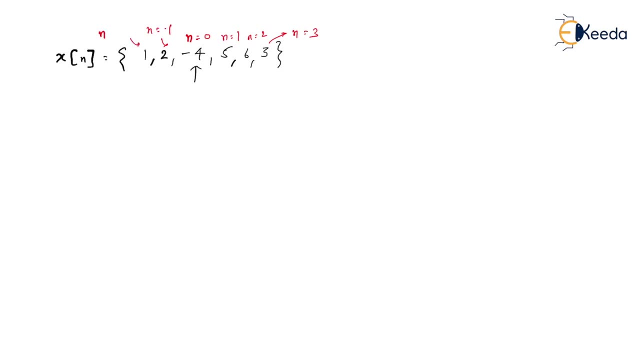 2 is present at n equal to minus 1, and 1 is present at n equal to minus 2. so you should always start with from extreme left position sample. so now i can write x of n equal to n. first of all, amplitude is plus 1, coefficient is plus 1. i can write del of n minus 2. 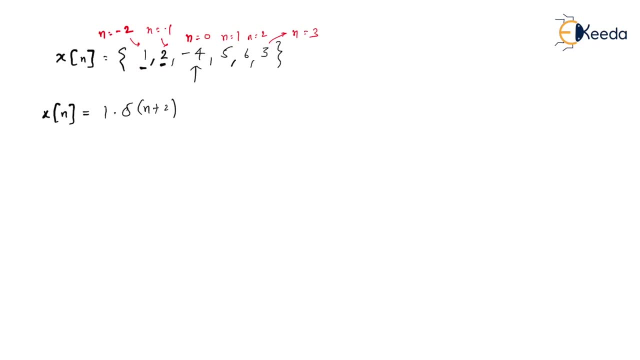 means i have to write plus 2 here. then coefficient is plus 2 del of n, plus 1. then at n equal to 0, amplitude is minus 4. therefore coefficient is minus 4 del of n because it is present at n equal to 0 position. then amplitude is 5, then i. 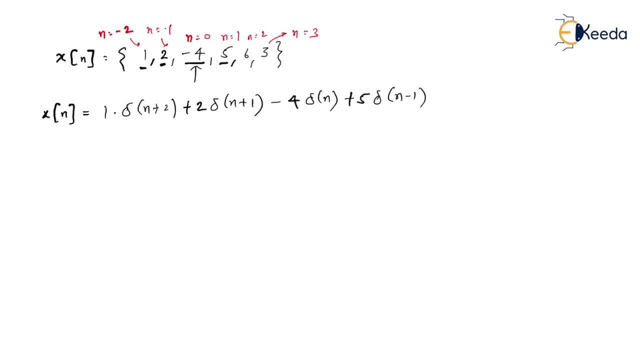 suppose to write plus 5 del of n minus 1. for n equal to 1, then we have amplitude 6, so i'll say plus 6 del of n minus 2, and last you are having an amplitude equal to 3. you write 3 times del of n. 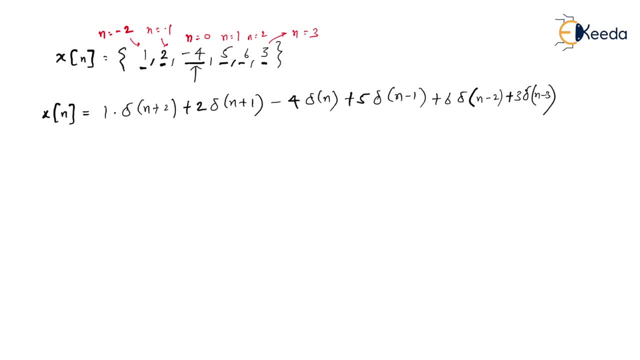 n minus 3. is that right? so now i'm just doing little modifications in the same. if you observe carefully, this minus 4 is nothing but x of 0, am i right? because x of n at n equal to 0 is minus 4.. i can replace this 5 with x of 1. i can replace 6 with x of 2. i can replace 3 with x of 3. 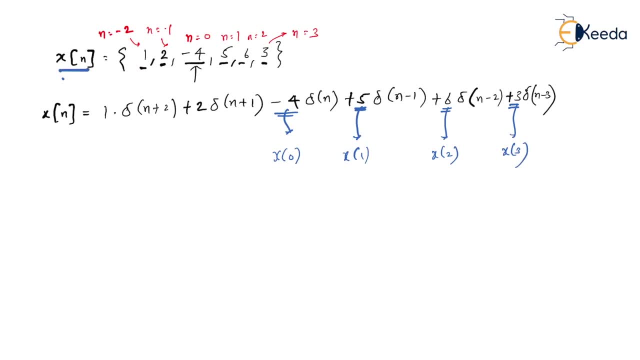 x of 3 means x of n at n equal to 3. as you can see, x of n at n equal to 3, it is 3, or x of n at n equal to 0, it is minus 4.. so this 2 is a coefficient which is nothing but x of minus 1 and this 1. 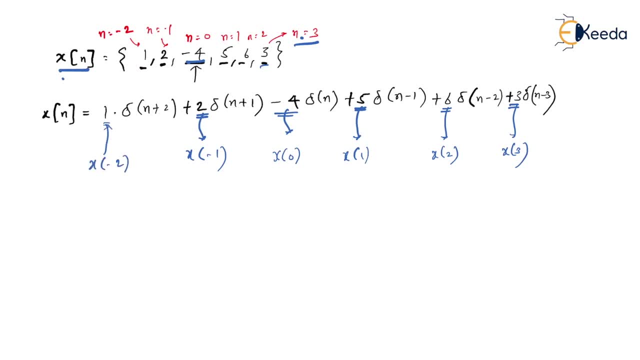 is nothing but x of minus 2.. so i'm rewriting x of n, x of minus 2, dot del of n plus 2 plus 2.. i should replace 2 with x of minus 1 only. so x of minus 1 del of n plus 1. 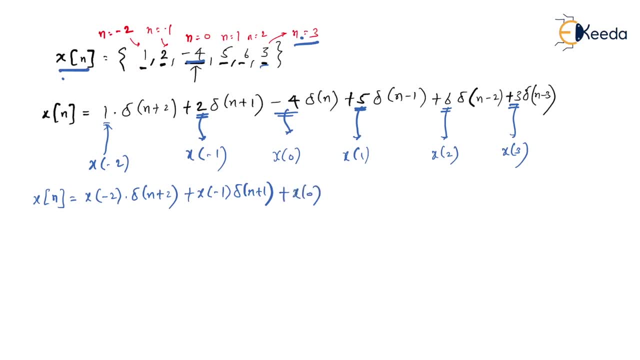 plus x of 0. okay, you can write plus here, because value of x of 0 is minus 4. so ultimately it will become minus 4, only del of n plus x of 1, del of n minus 1 plus x of 2, del of n minus 2 and finally, 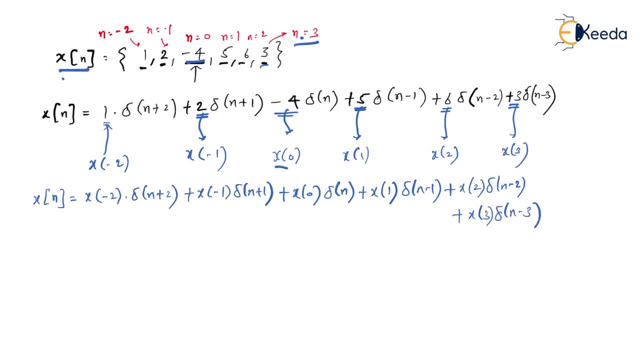 plus x of 3 del of n minus 1.. is that, right now, if you observe carefully, here it is minus 2, then it is plus 2, here it is minus 1, then it is plus 1. if it is 0, then nothing is present. here. if it is 1, it is minus 1, if it is 2. 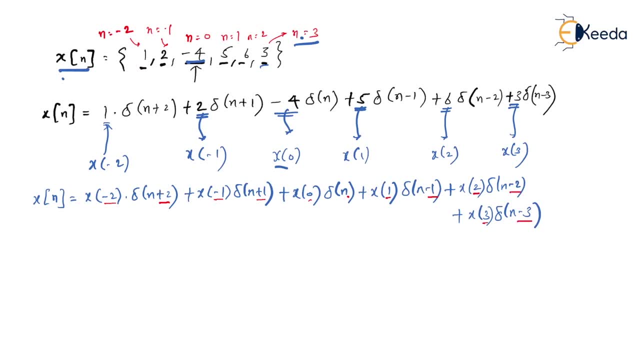 it is minus 2. if it is 3, it is minus 3.. what i really mean to say is: i need to write it in a shot so i'm able to do this. if you see, it is actually following a common format everywhere. is that right? so it is following a common format everywhere. 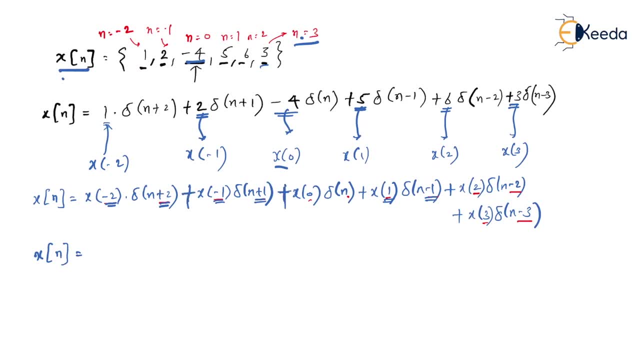 and then it is summation of all together. so i can write some summation symbol here and if you see the value of variable here and here it is same. here and here it is same. so i can replace with another variable, let's say k. so i can write this as x of k, dot del of now. 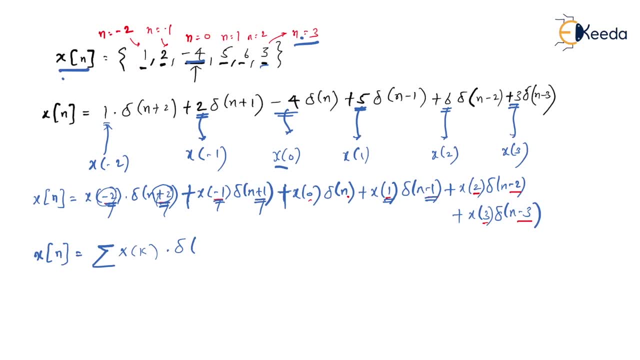 if this is minus 1.. then this is plus 2.. so if i say plus k here, i need to say it is minus k, so i can write n minus k. is that right? and as you can see the value of k: okay, the starting limit is minus 2. 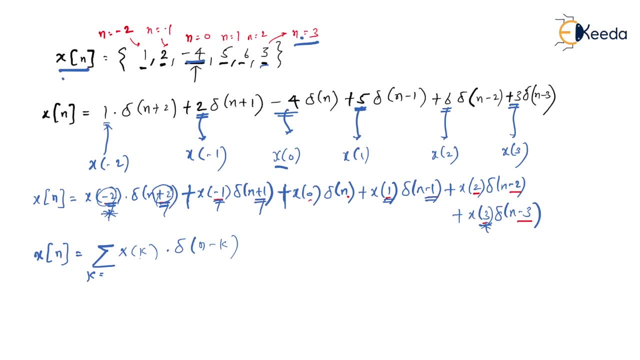 and the highest limit is plus 3.. so i'll be varying my k from minus 2 to plus 3.. so i can represent my x of n in the form of this, that is, x of n is equal to summation, where k is varied from minus 2 to plus 3. x of k, dot, del of n minus k. but do you think that every 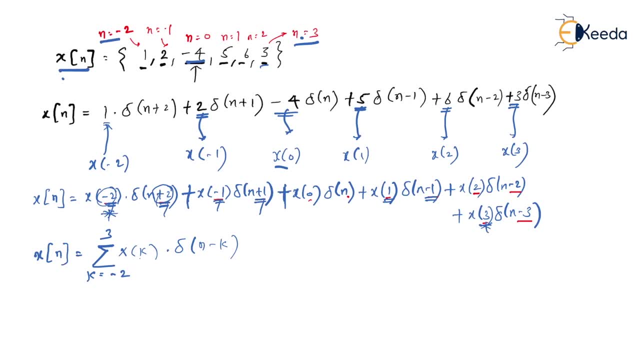 time. your discrete time sequence is starting with n equal to minus 2 and ending at n equal to plus 3. no, it is not so. it is going to vary depending upon the size of signal, depending upon the length of signal. so if the signal varies, this expression is going to vary.